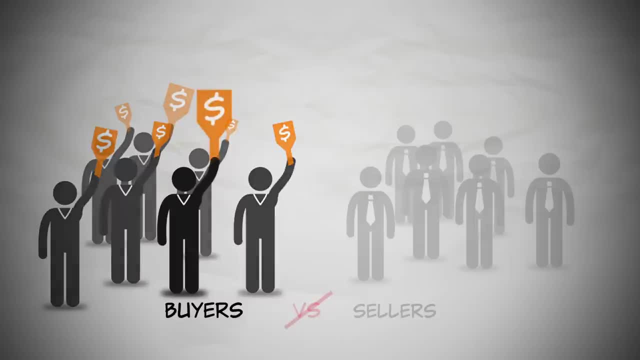 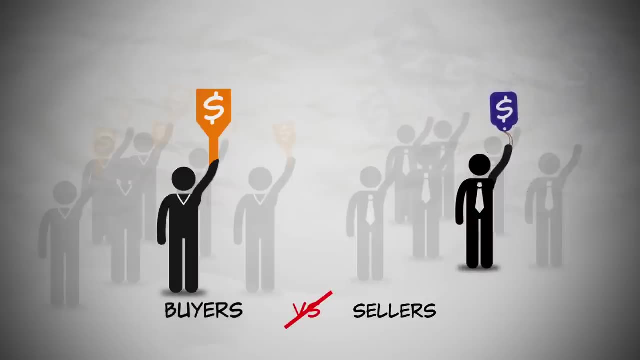 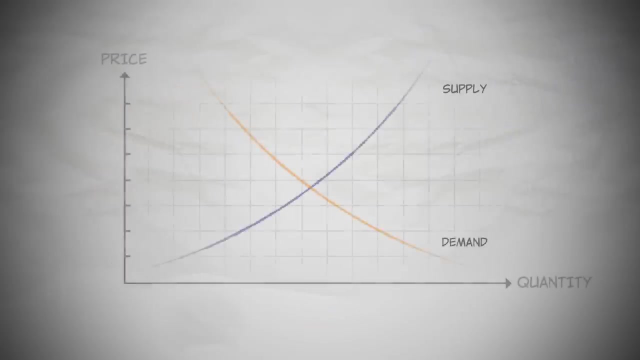 buyer obtains goods by bidding higher than other buyers, And sellers compete against other sellers by offering to sell at lower prices. Think about it At an auction: the buyer with the highest bid gets the item and the seller with the lowest price makes the sale. So let's say the price of oil is: 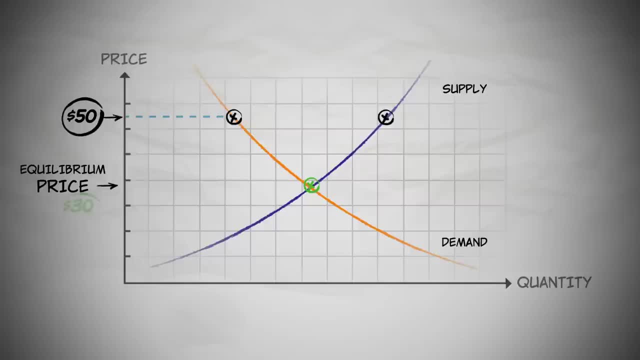 currently 50 bucks a barrel. That's above the equilibrium price of 30 dollars a barrel. At 50 dollars a barrel the quantity supplied is more than the quantity demanded. So we say there is a surplus. So what happens? It's sale time. When there's a surplus, sellers can't sell as much as. 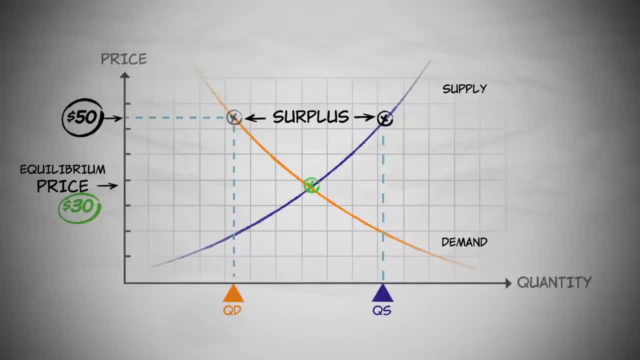 they would like to at the going price. So sellers have an incentive to lower their price a little bit so they can out-compete other sellers and sell more. The price will continue to fall until the quantity demanded is equal to the quantity supplied. So the price will continue to fall until. 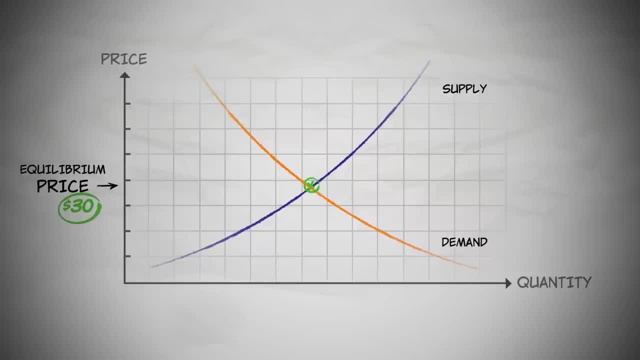 the quantity demanded is equal to the quantity supplied. So the price will continue to fall until an equilibrium is reached. Now let's say the price is less than the equilibrium price, Say 15 bucks a barrel. At 15 bucks a barrel, the quantity demanded exceeds the quantity supplied. A 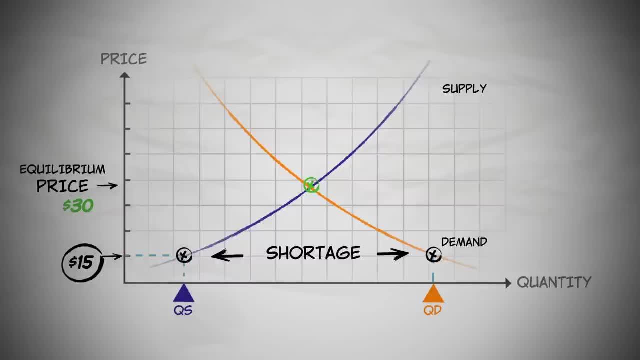 shortage. And what happens now? When there's a shortage, buyers can't get as much of the good as they want at the going price, So they compete to buy more by bidding up the price. Now, since buyers are easy to find, sellers also have an incentive to raise the price. The price will 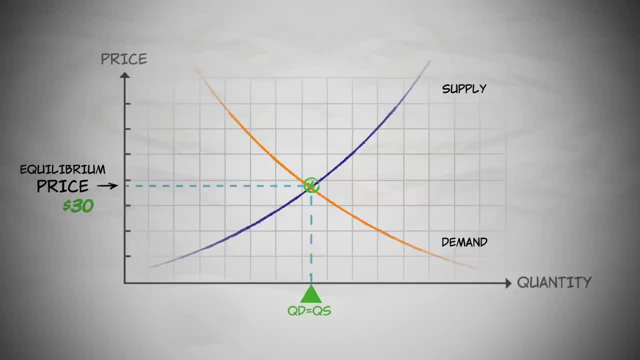 continue to rise until quantity demanded is equal to the quantity supplied. So the price is equal to the quantity supplied and equilibrium is reached At any price other than the equilibrium price. the incentives of the buyers and sellers push the price towards the equilibrium price. Only the equilibrium price is stable. Now let's take a deeper look at the market equilibrium. 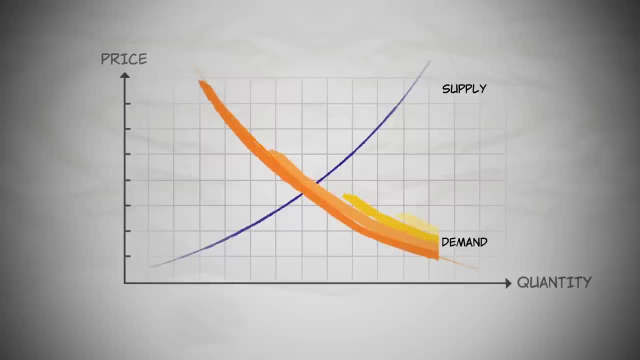 and some of its properties. Remember that there are many different users of oil and many different uses for oil, each with substitutes, alternatives and values. At any specific price of oil, there's a group of buyers who value oil enough to demand it at that price, And as the price changes, so do the buyers, and 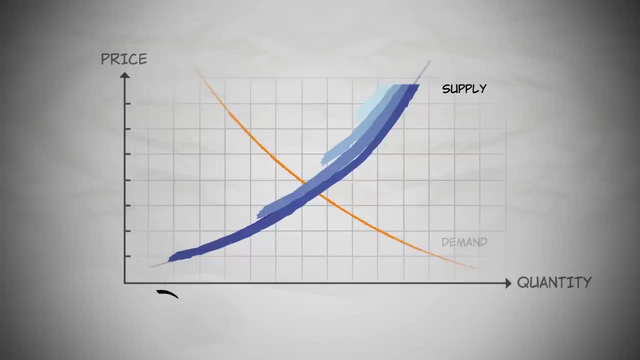 their uses. On the supply side, at each price on the supply curve, we're looking at a group of suppliers whose cost of extraction is low enough to be profitable. at that price, At the equilibrium price, these higher value groups are the buyers and these lower value groups